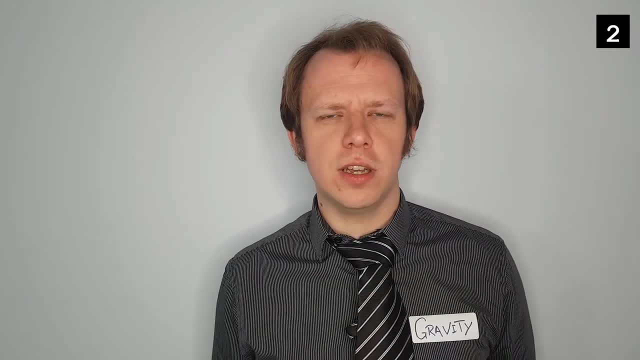 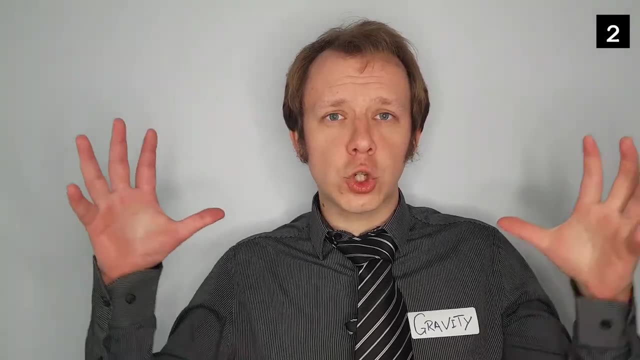 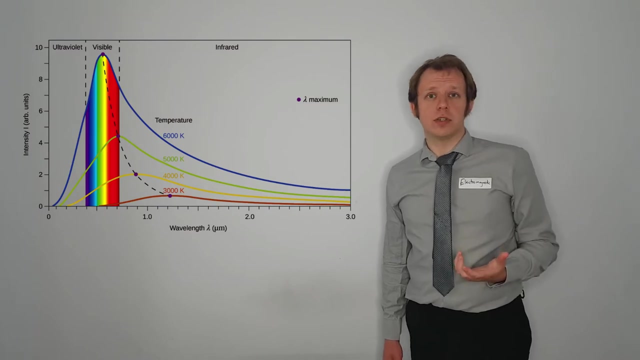 But when they're contracting, they're losing gravitational potential energy. This gravitational potential energy is converted to heat, and so as our protostar contracts, it gets hotter. As they get hotter, they will emit more light, acting as black bodies. So the hotter they get, they'll both emit more intense light and light of shorter and shorter weight. 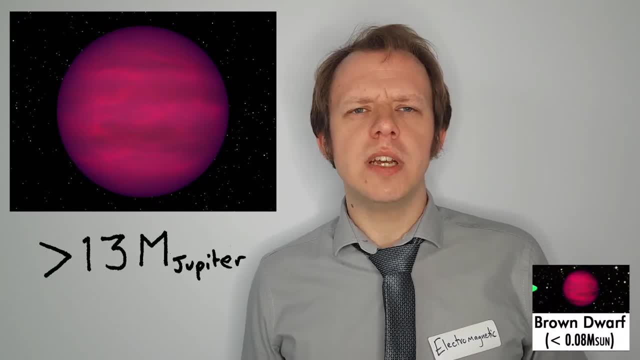 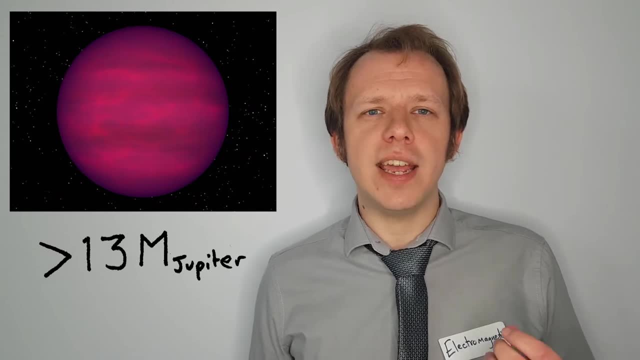 This is because of the mass of Jupiter. Above about 13 times the mass of Jupiter, they'll be producing enough radiation to be classified as a brown dwarf. Now, this still isn't a star, but it is emitting a lot of infrared radiation and a little bit in the visible spectrum. It's called a brown. dwarf because of the low intensity of the light that it's producing and because it's very small For more massive protostars, and we're talking here about at least 0.08 solar masses. as they contract, they reach temperatures of at least 10 million kelvin. 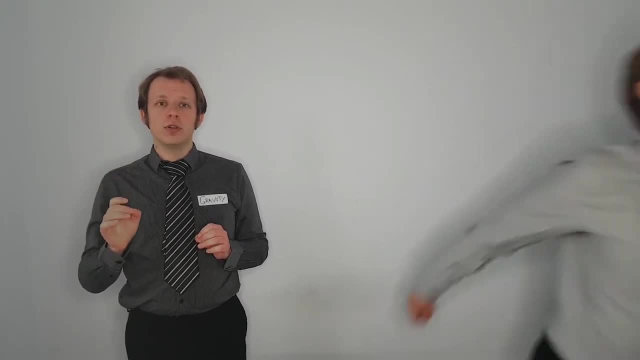 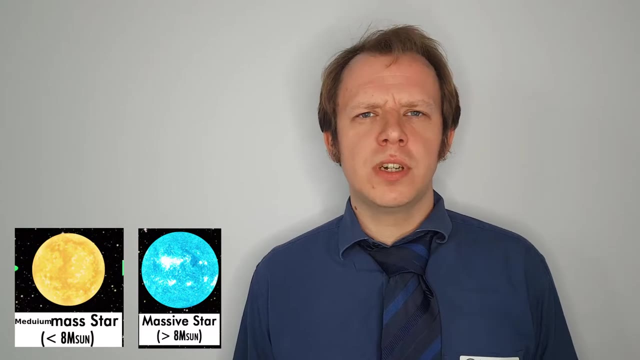 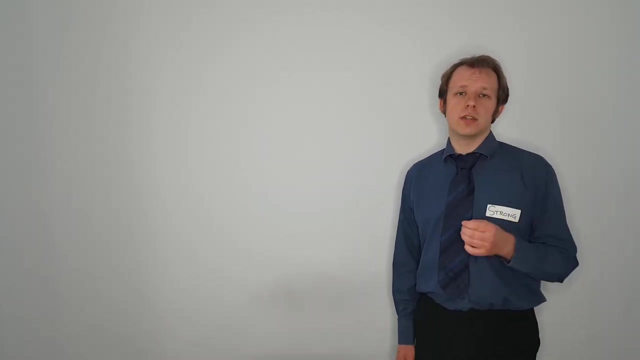 And this is enough energy for our protons to overcome the electrostatic repulsion between them. This is the start of nuclear fusion. At this temperature, hydrogen can fuse into helium and finally we have a true star. And there are a couple of different ways that stars do this. 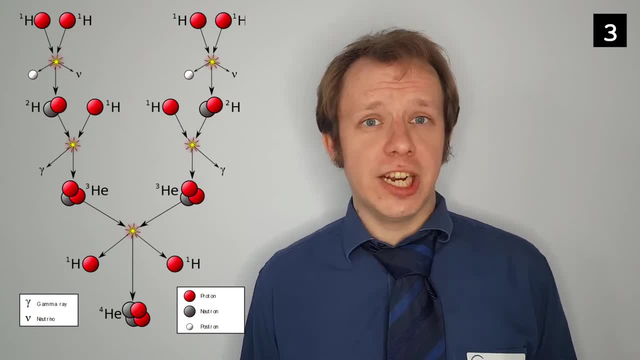 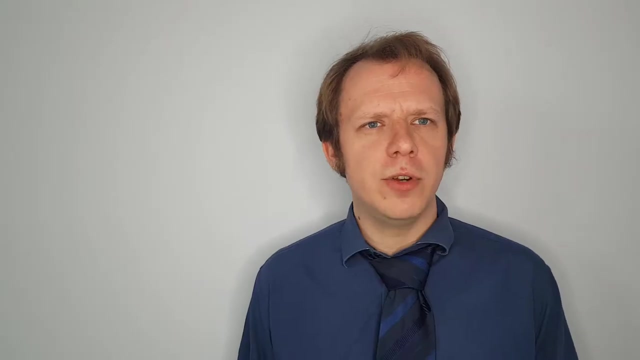 The first is the proton-proton chain or the PP chain. In this we have individual protons combining together to form a heavier helium nucleus. With two of the protons emitting positrons come neutrons, living or stable nucleus. The final helium nucleus produced has a lower mass than the nucleons that we 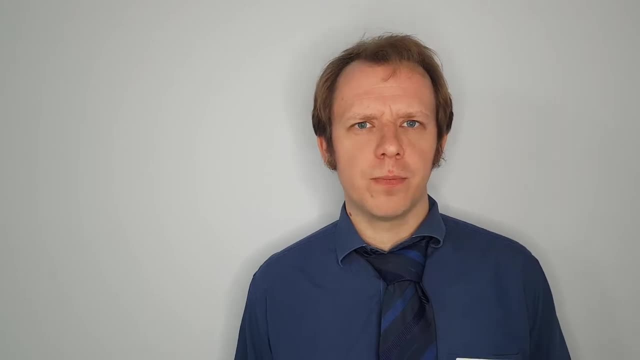 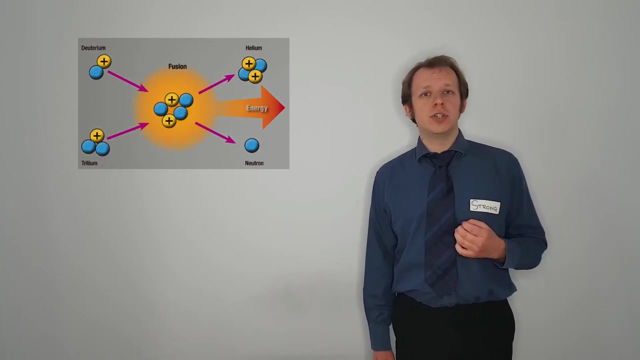 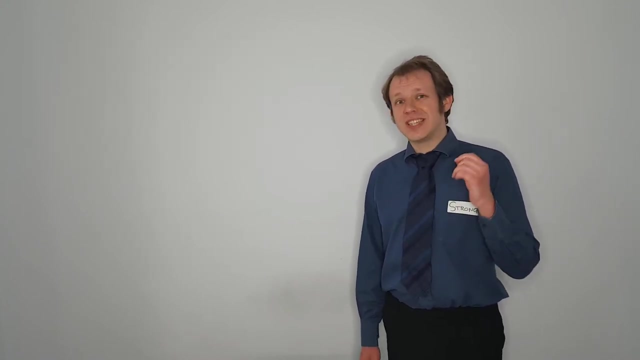 started with because it has a higher binding energy per nucleon. This means that there is energy released during each one of these fusion reactions That every helium nucleus produced. about 25 mega electron volts are released. Our alternate path is something called the CNO cycle. 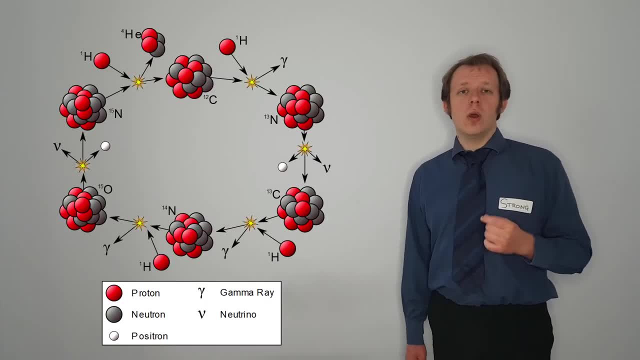 We can see that, although this nucleus is changing throughout this cycle, once that alpha particle, once that helium nuclei is released, we are back to the carbon that we started with. So in this case, the carbon is released. So, in this case, the carbon is released. 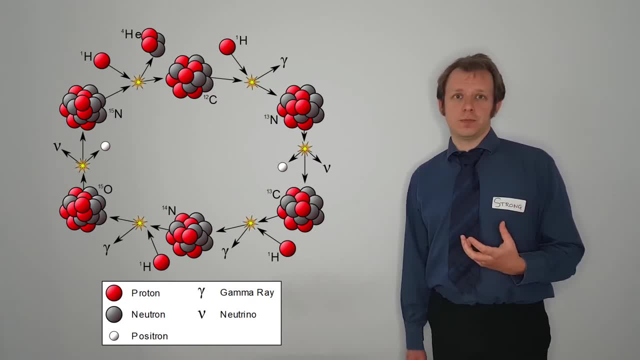 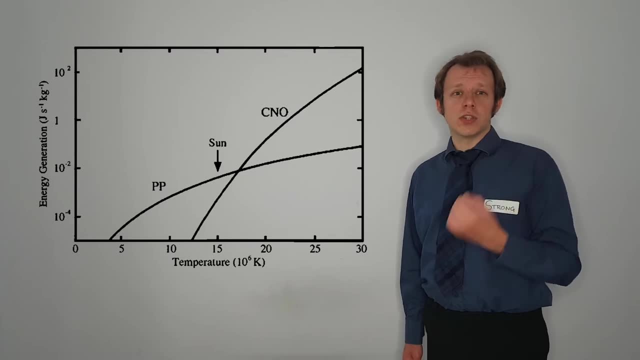 So in this case the carbon is released. The carbon is not used up, it is just acting as a catalyst. Now the CNO cycle becomes much more efficient at higher temperatures. So for a star the size of our sun it will not really be producing very much energy at. all through the CNO cycle. It does need to be a larger star to have that increase in mass, to have that higher temperature. Both the PP chain and the CNO cycle all release energy and this energy is now able to counteract that gravitational contraction and an equilibrium is reached. 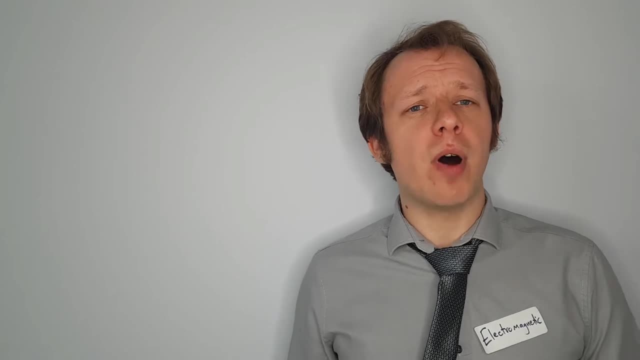 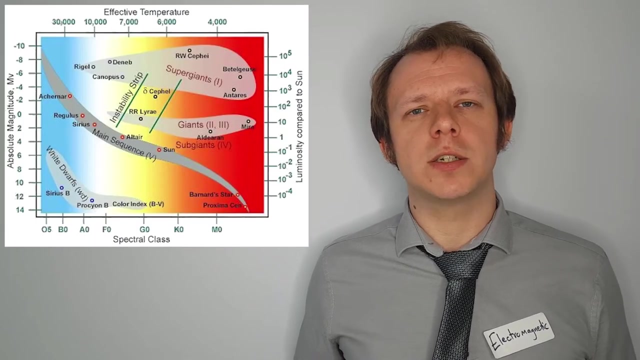 We've classified stars according to their brightness, their absolute magnitude and by their colour, which tells us about their temperature. We can combine both of these classifications on something called a Hertzsprung-Russell diagram. Hertzsprung and Russell actually came up with a very similar way of classifying it independently. 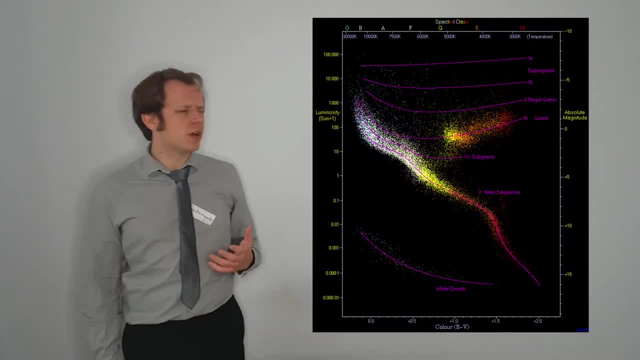 and the diagram was therefore named after both of them. Now, one of the things that we notice on it is that the stars are not randomly spread about. Most of them, in fact, go along this line in the middle, So the stars are not randomly spread about. 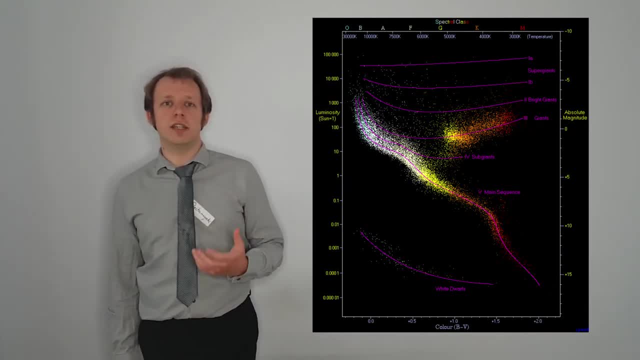 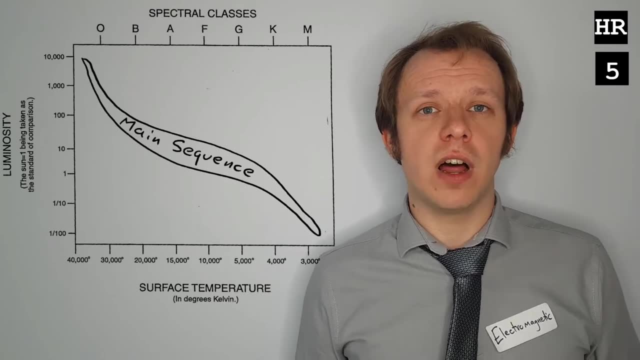 Most of them, in fact, go along this line in the middle, And this is referred to as the main sequence. It was originally classified by using this diagram. however, as our understanding of the life cycle of stars has improved, we've seen this is the hydrogen burning phase of 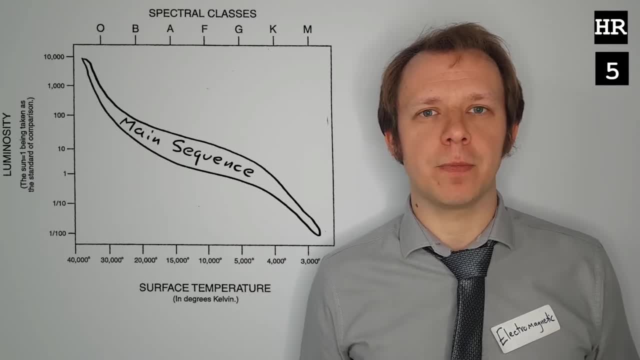 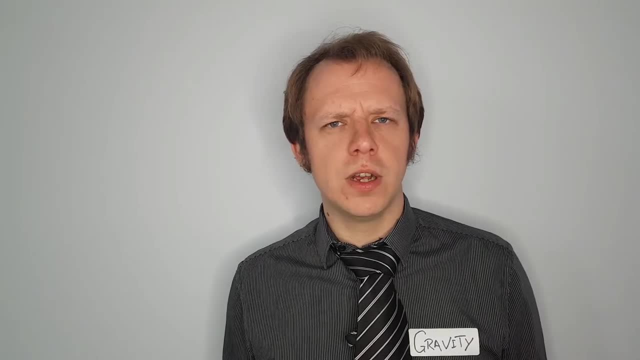 a star, This is the main part of its lifespan. Now the time on the main sequence is very different for different stars. Now you might assume that the more massive a star is, the more fuel it has and the longer it will survive. 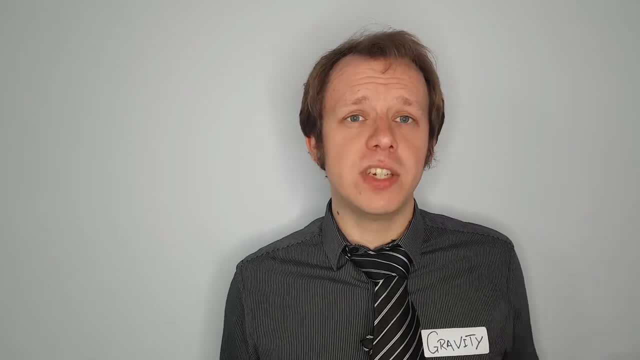 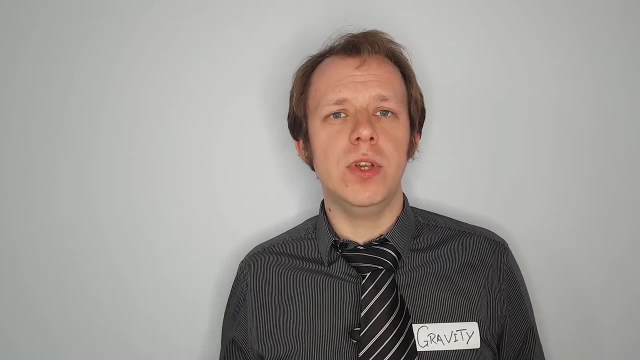 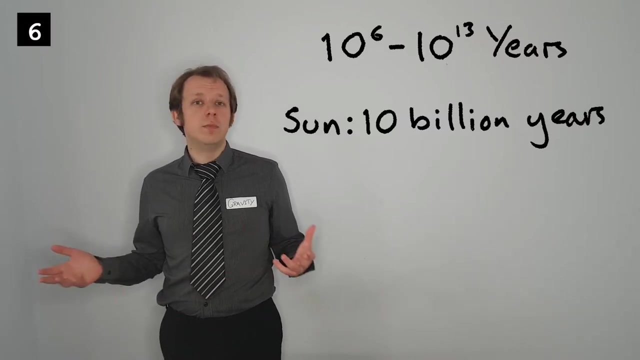 But in fact the opposite is true. The more massive a star is, the more gravitational potential energy is converted into heat. The hotter it burns, the quicker it uses its fuel and the shorter its lifespan. The very largest stars can burn themselves up in a few millions of years. 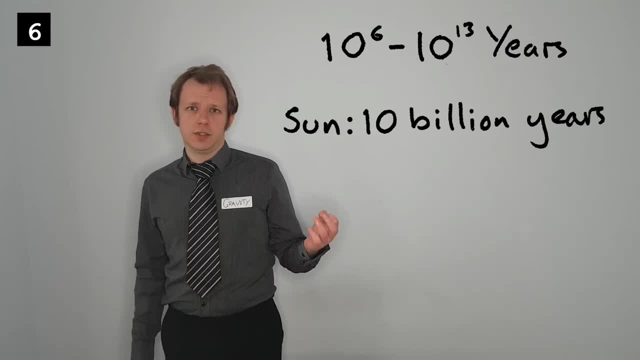 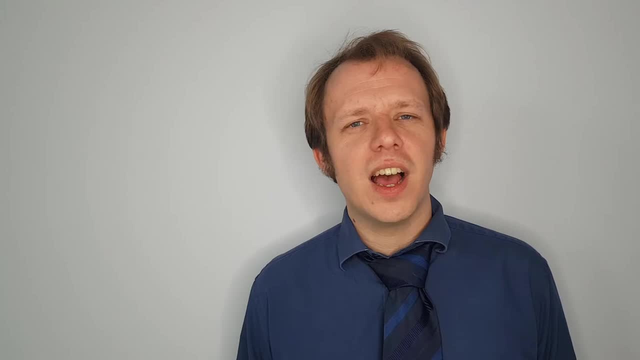 Whereas the smallest might last trillions, Many orders of magnitude longer than the lifespan of the universe so far. Eventually, there'll no longer be enough hydrogen in the space of a second star, so this is our busiest of all time. That's the Big Bang Theory. 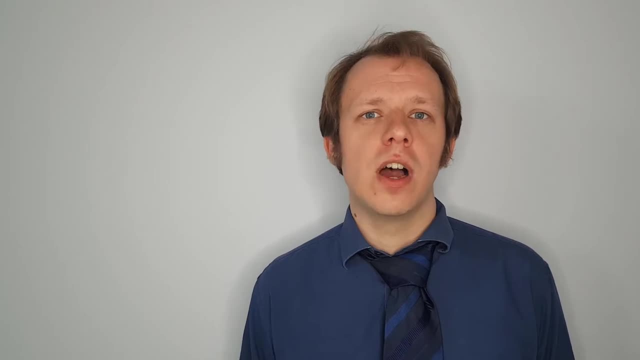 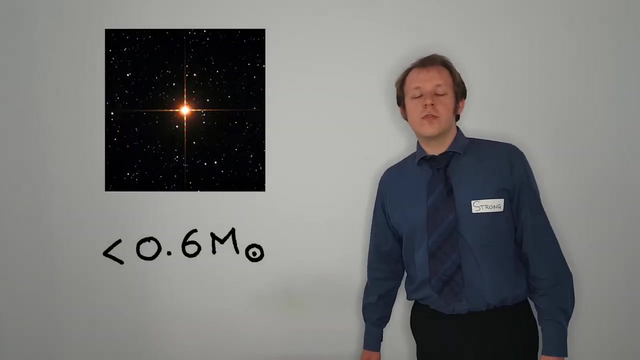 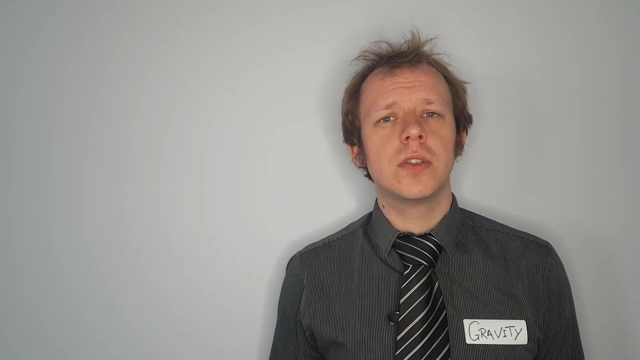 core to sustain nuclear reactions and the star will end its time on the main sequence. But what happens next depends very much on the mass of our star. The very smallest stars take a vast amount of time to use up all their fuel Without fusion to support it. the star 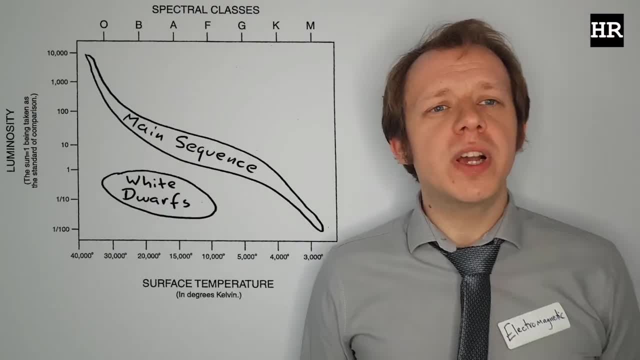 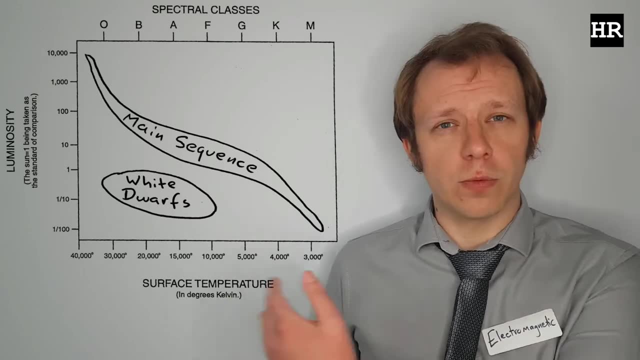 will contract, getting hotter in the process. Because these stars are very small, they will have a low brightness, but the surface temperature is very hot, so they are a sort of white colour. This leads them to be classified as white dwarfs on this area of the Hertzsprung-Russell. 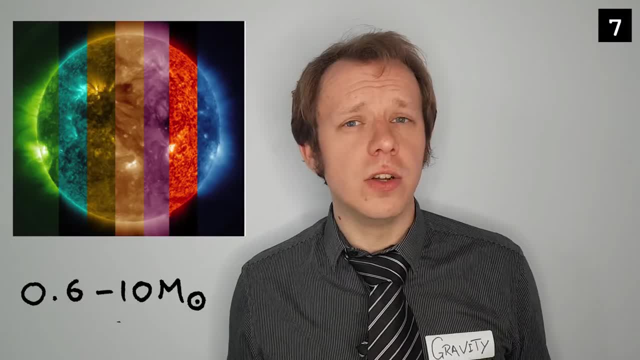 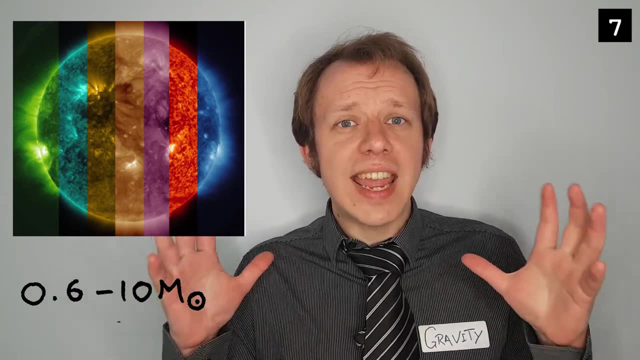 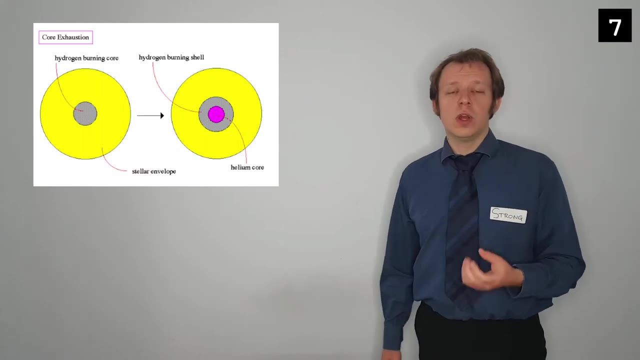 diagram For mid-sized stars, and that includes our Sun. once there is no longer enough hydrogen for fusion, that core will start to contract again And as that helium core contracts, it will get hotter and hotter. Although there is no fusion inside this helium core, that hotter temperature causes the hydrogen around. the core to start fusing, And even though the core itself has been shrinking. this is because the fusion in the outer layers of the star in fact causes the outer layers to expand. As these stars expand, the energy is more spread out, and so the temperature. 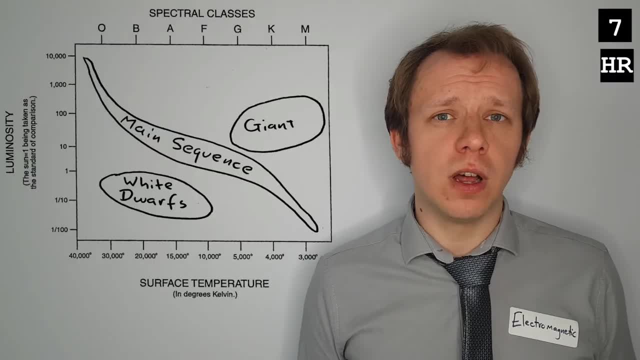 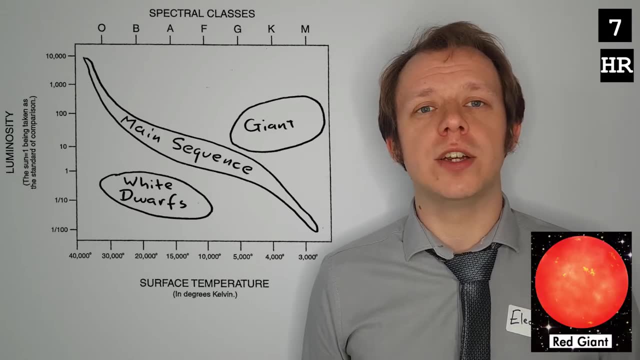 decreases and so they become more red colour. But because they are so large they are still producing a lot of light, so they are pretty bright. So they go on this area of the Hertzsprung-Russell diagram and they are known as red giants, And because the helium produced in those outer layers is more dense than the hydrogen surrounding it, it will sink to the core, making the core heavier, making it contract more and making it hotter. And now the core is massive enough to reach a temperature where helium fusion can start. Everything else we've been talking about has been on a timescale of millions or billions. 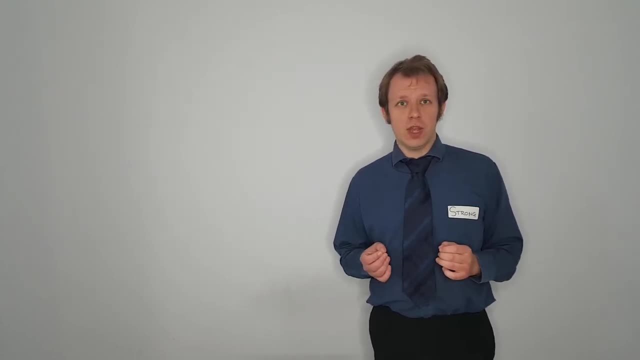 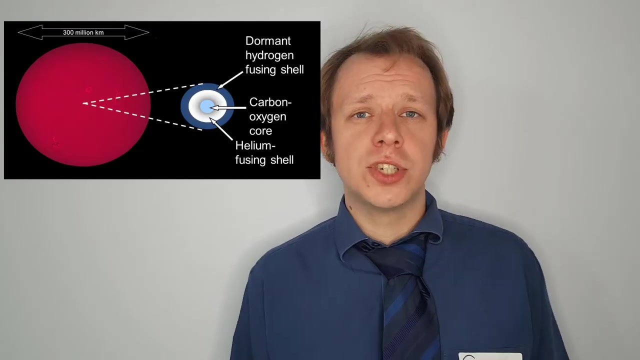 of years. This happens in a matter of days. It's known as the helium flash and leaves behind a core of mostly carbon and oxygen. Although the carbon and oxygen in that core cannot fuse, the core reaches a high enough temperature that the helium surrounding it. can begin to fuse, And the hydrogen surrounding that can also fuse, and so we remain in our red giant phase. During this phase, the energy released causes intense solar winds that send matter from the star out into the surrounding system. These can end up being larger than the system. itself and is known as a planetary nebula. Now these stars are not heavy enough to reach the temperatures necessary for the next stages of fusion, and so they continue to contract. Contraction is halted by a quantum effect called a Lagrangian effect. 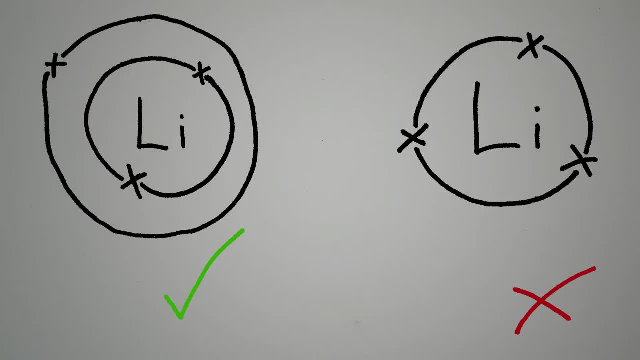 The Lagrangian effect is a quantum effect called a Lagrangian effect. These thermonuclear forces, where water between levels matches the temperature of know extreme maximum, are forced against each other and create electrons caused by these electrons that pass a random temperature of 1 to 10 Kelvin semitissa for them to share. 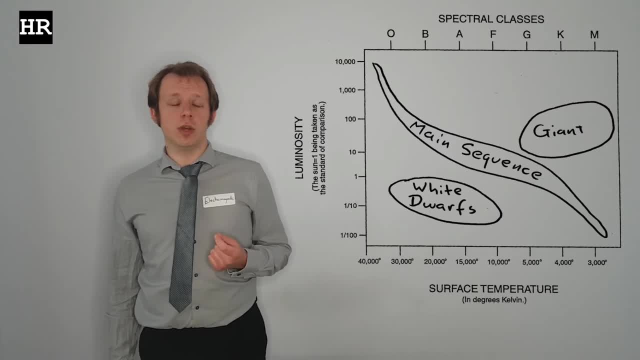 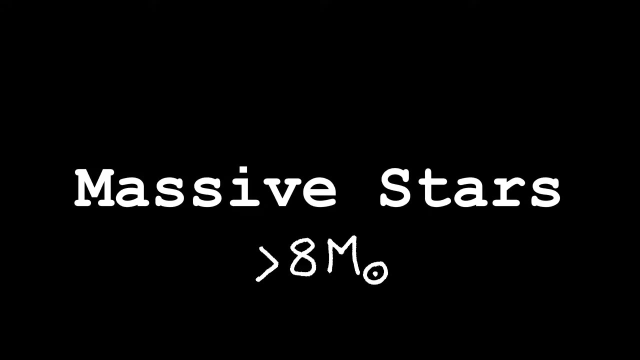 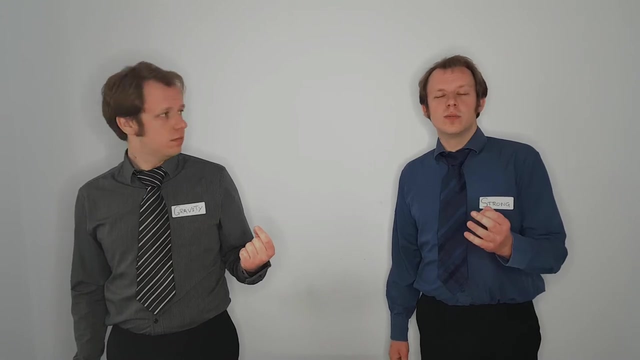 But these electrons can not communicate this gas. They don't. But what happens at the end of this state of fusion is what can happen, 같아요. As we've said, more massive stars burn at higher temperatures and have much shorter lifespans. 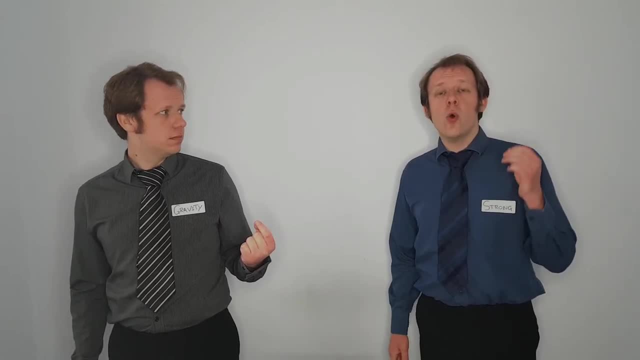 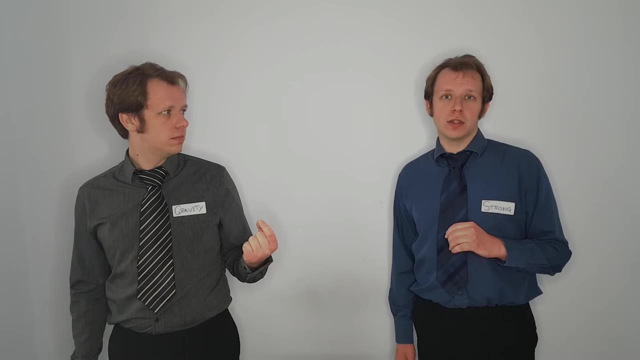 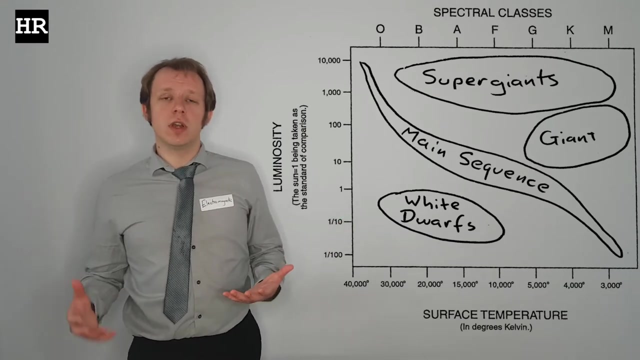 By the time it reaches the stage where it's burning the hydrogen shell, the core is already hot enough to be burning helium. So these more massive stars will never get the helium flash that we have with lower mass stars. In the same way that our red giants became larger with a lower surface temperature, these stars are even larger, And so we refer to these as our super giants. With no fusion to support it, the core will contract, getting hotter and hotter, causing the fusion of heavier elements until those run out. Again, with no fusion to support it, the core will start to contract again, getting hotter. and hotter, causing the fusion of heavier elements. until those run out And with no fusion to support it, the core will again contract, getting hotter and hotter, getting hotter and hotter, causing the fusion of heavier elements Throughout each stage of this nuclear fusion. 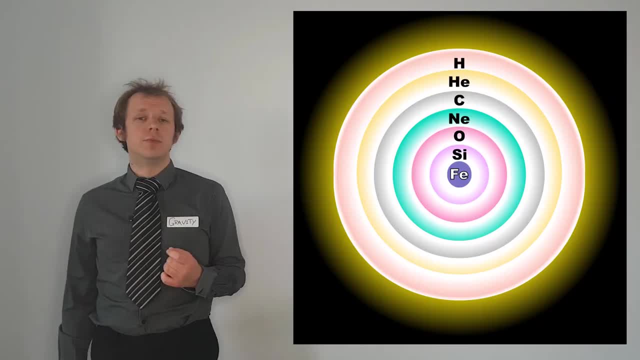 we've been burning heavier and heavier elements. As the heavier elements are produced, they will sink, leaving the layers kind of like an onion, with the densest at the center working their way out to the lightest. This has been fine so far. because, as we have gone up the periodic table, the binding energy per nucleon has increased. so we are getting more and more stable nuclei and releasing energy with each fusion reaction, If we remember the graph that we looked at showing the binding energy per nucleon. it reaches a peak at iron. This is the most stable nuclei and we cannot fuse heavier elements without absorbing energy. They're essentially endothermic rather than exothermic, so they're not gonna be able to balance out the gravitational forces of the star. 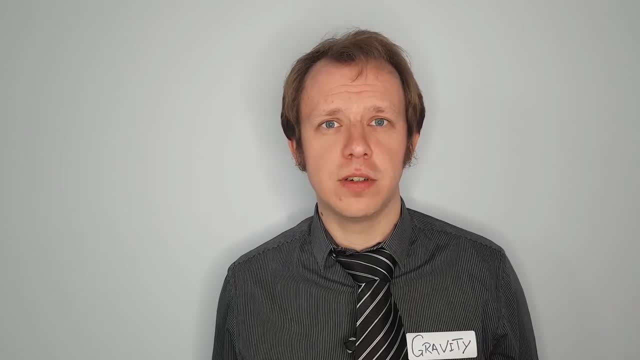 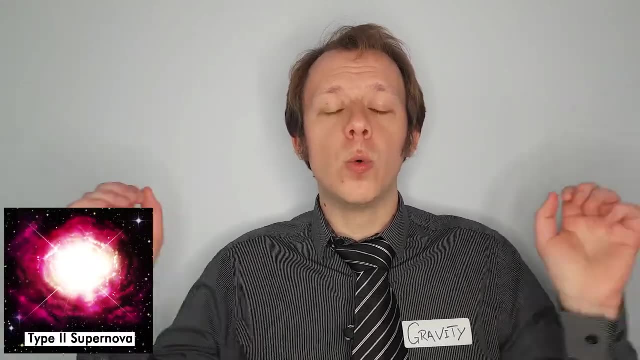 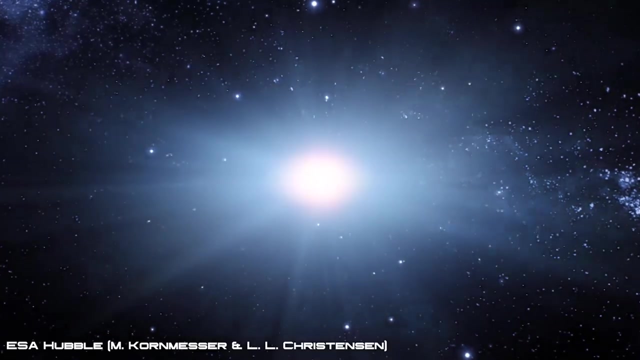 With no fusion to balance the weight, the core will start to collapse. As the core collapses, the layers around it will also fall in on it, compressing more, rebounding off that core and releasing a vast amount of energy. Enormous forces and temperatures are unleashed. 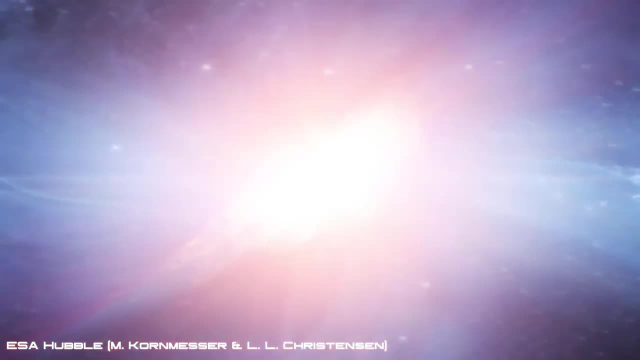 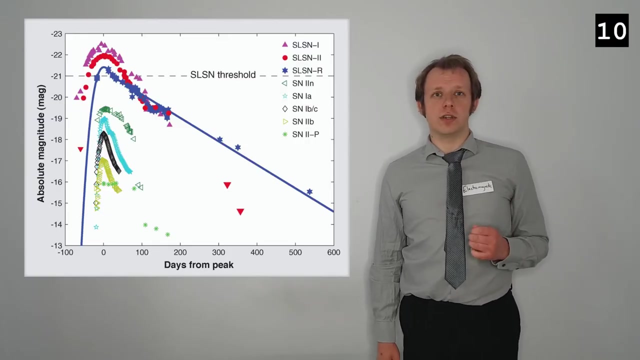 and here there is enough energy to form elements heavier than iron. This output of energy vastly increases the absolute magnitude of the star. For a very short time it outputs much more energy than at any other stage of its life. A single supernova can be producing as much light. 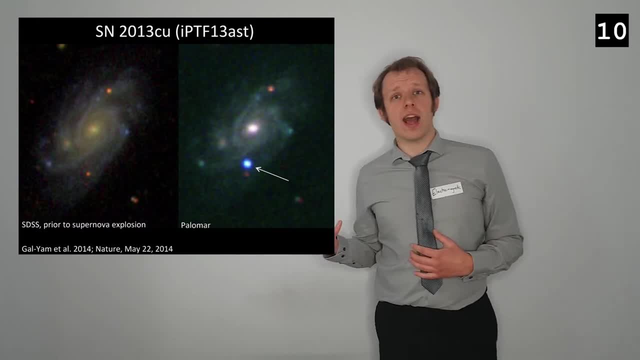 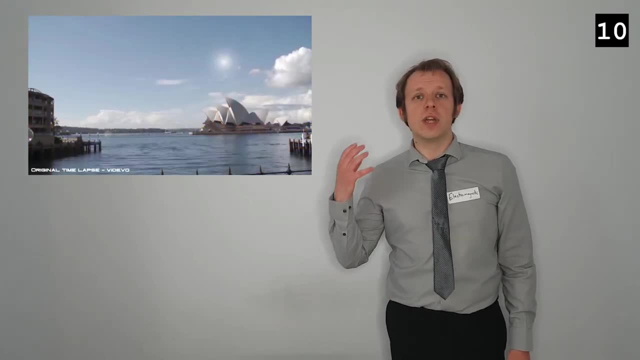 as pretty much this entire galaxy it's in. In fact, if there was one in our galaxy, we would be able to see it day and night. It would be comparable to the sun And, of course, at these vast energies, we're also producing more and more. 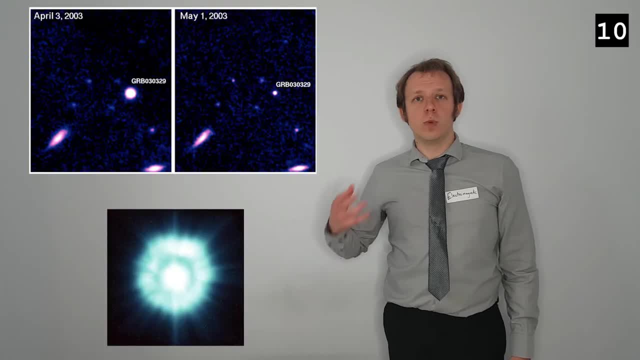 of our higher frequency ionizing radiation, We get a gamma ray burst from supernovas. This vast outpouring of gamma rays is a clear sign that a supernova has happened. It's one of the things that astronomers love, Although, of course, if one happened too close to Earth. the intensity of the gamma rays would be enough to wipe out all life on our planet. Now, after this explosion, the outer layers have been exploded off into a supernova remnant. What's left at the core can be a couple of different things. depending on the mass of the star. We've seen white dwarfs supported by the electron degeneracy pressure, but these stars are much more massive. The core left behind is even more dense than a white dwarf. The gravity now is strong enough to overcome the degeneracy pressure. 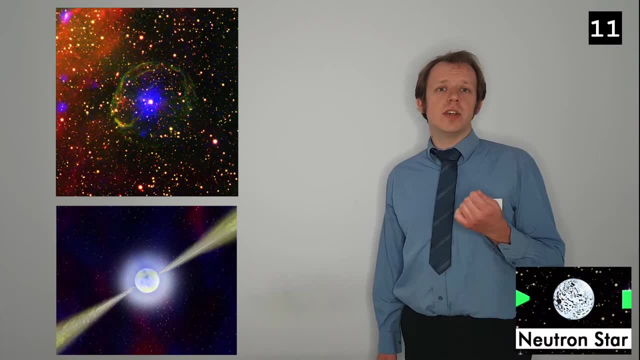 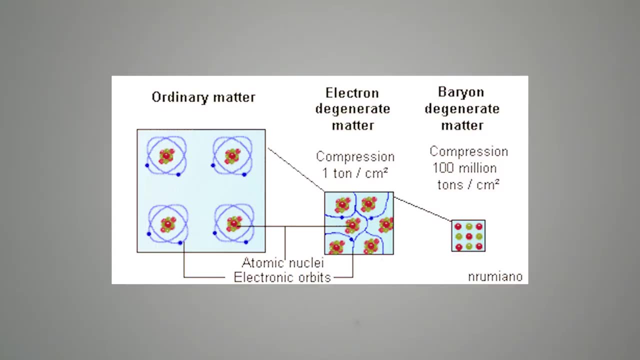 and the protons and electrons combine to form neutrons, leaving us with an object made almost entirely of neutrons and of a pretty similar density to a nucleus itself. This is another form of degenerate matter, with further compression resisted by neutrons, obeying the Pauli exclusion principle. 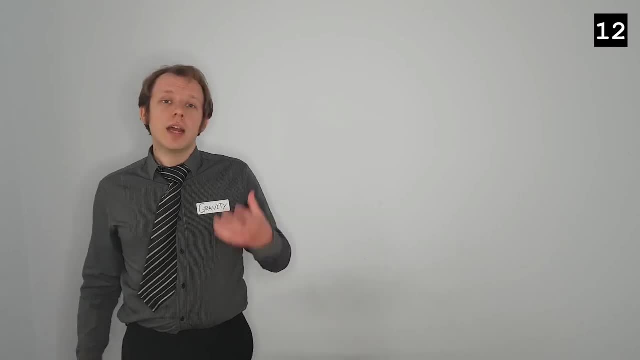 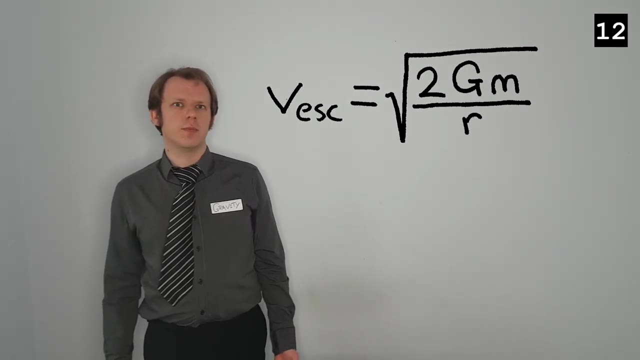 Now these neutron stars: we know they have a very high mass and because they are so dense they also have a very low radius. Now, if we look at our formula for escape velocity, we can see that increasing the mass and decreasing the radius,